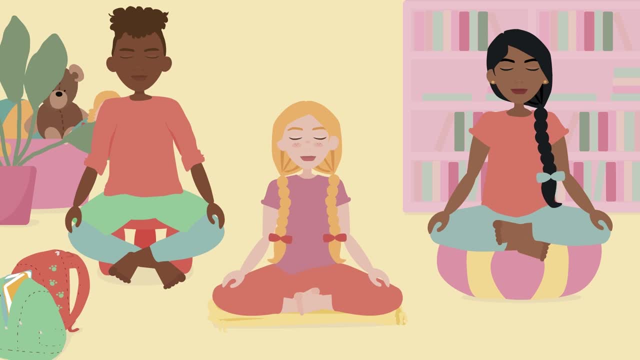 through your nose and breathe out through your mouth. Really try to focus on your breath. Feel your belly and ribs expand as you slowly breathe in Deep breath in through your nose and breathe out through your mouth One more time: Deep breath in through your nose. 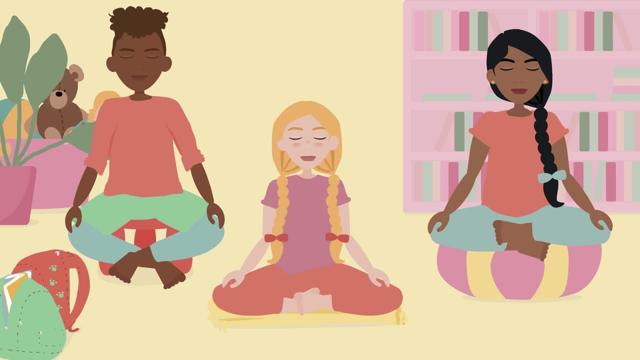 and breathe out through your mouth One more time. Deep breath in through your mouth. Your plançing will heal. Now that we have relaxed our minds, let's use our imaginations to transport ourselves to our happy places. Think of your favorite place in the whole entire world. 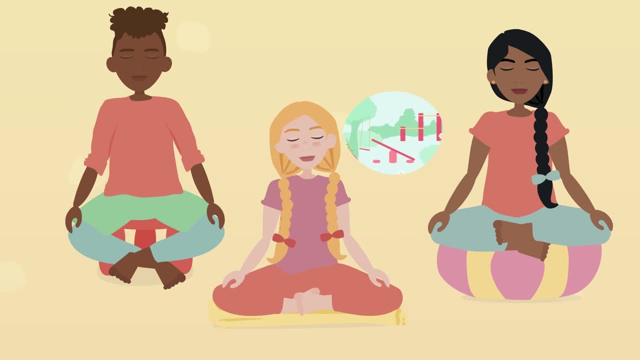 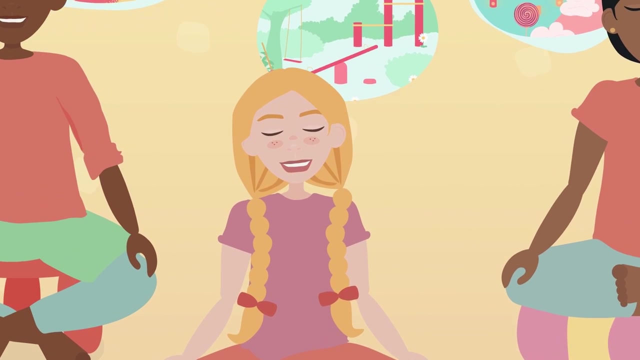 Maybe it's the playground or the beach, or a world you created entirely in your imagination. There are no wrong answers. This is your happy place and it will also tranquilize you throughout these 3 days. happy place Maybe it's a soccer field or the library, or even your grandmother's. 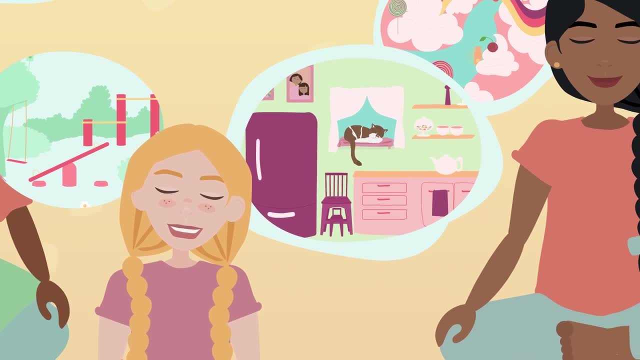 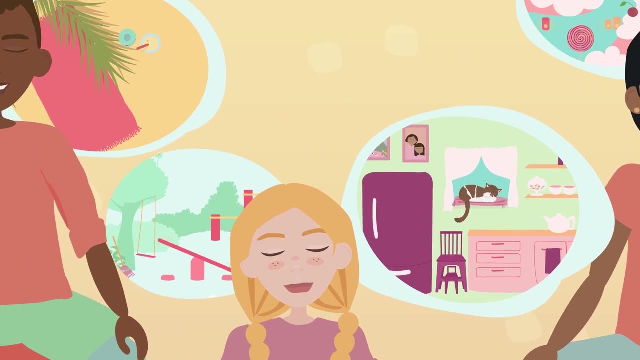 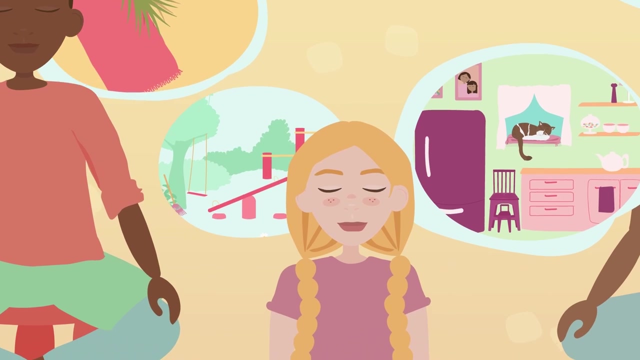 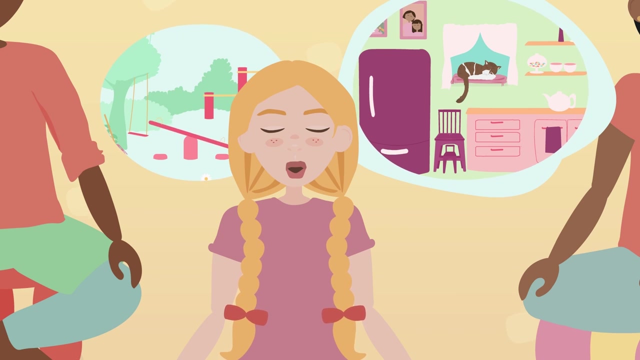 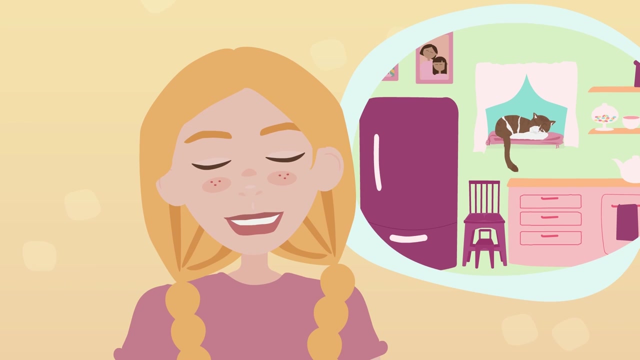 kitchen. Think of a place that makes you feel happy, calm and safe. Take a deep breath in through your nose and let it out. Your happy place is a positive space, so let's think about things that make you feel really positive and happy. 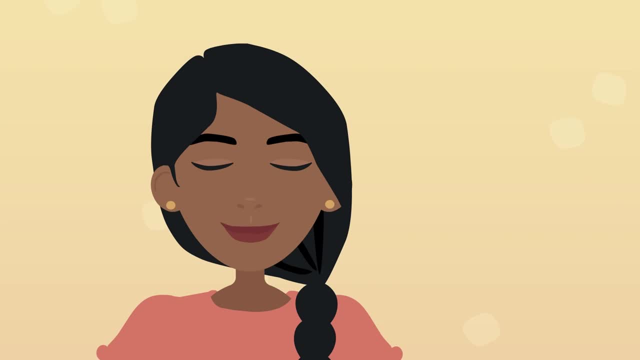 Think about something that makes you feel happy, calm and safe. Think about something that makes you feel happy, calm and safe. Think about something that you are really grateful for. Maybe it's your family or friends or teacher, Or maybe it's your favorite food. 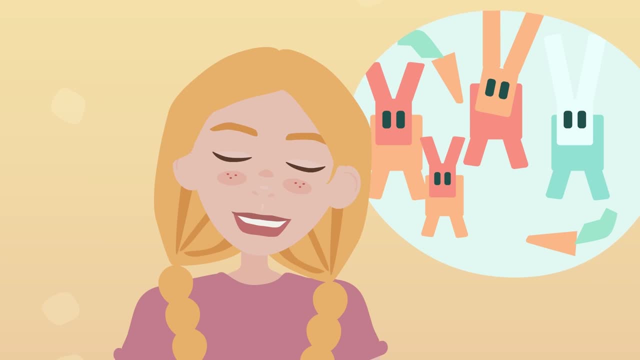 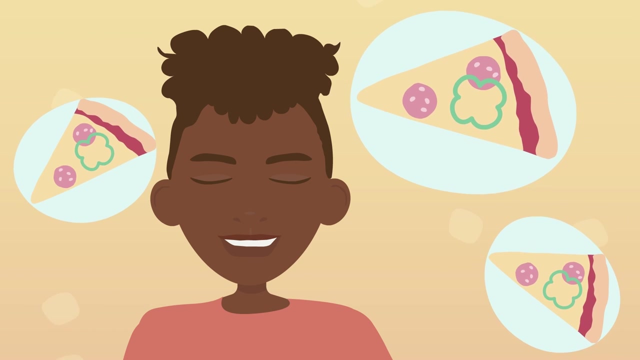 Or maybe it's animals, video games, books or even laughter. There are so many things to be grateful for. Choose one, or as many as you can, things you can think of that you are grateful for today. take a moment and think about how grateful you are for that thing. now think of something that. 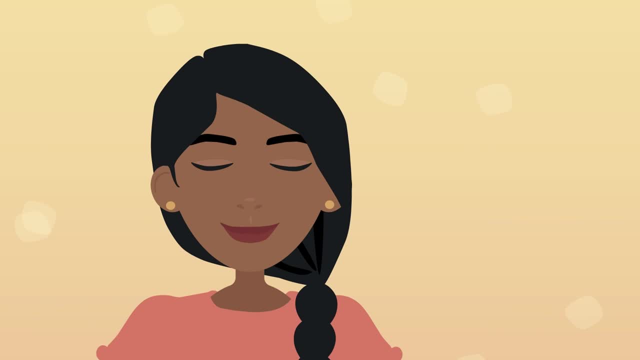 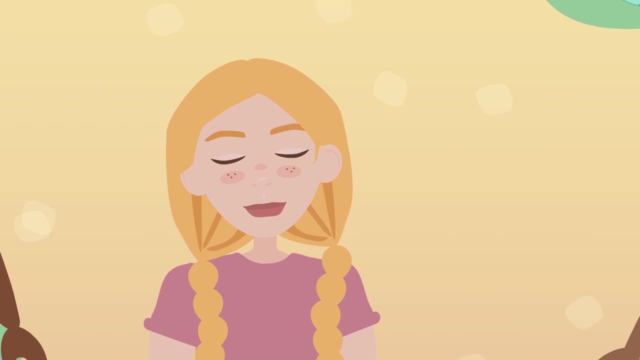 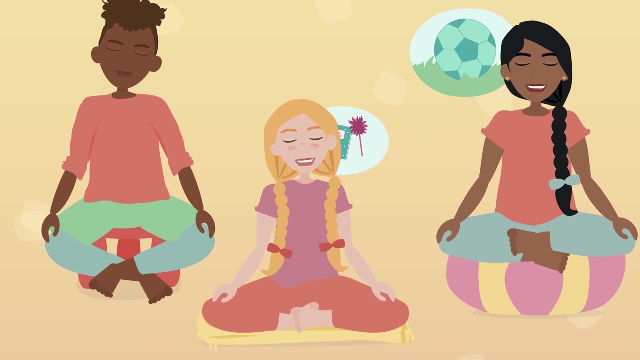 you are really excited to do today. maybe you're excited to go to soccer practice, or to learn something new, or to see your friends choose one or as many things you can think of that you are excited for today. maybe you're excited to use your new notebook, or to turn in a homework assignment you worked really hard on, or 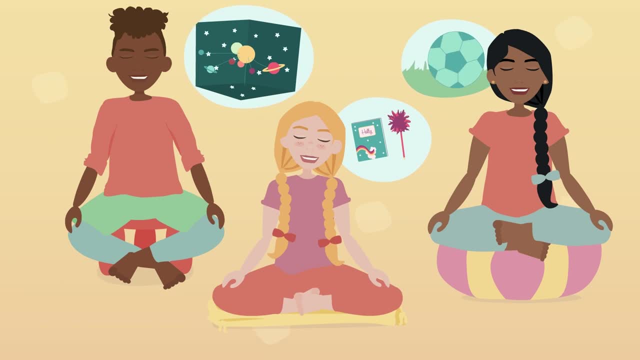 to eat your favorite sandwich for lunch. take a moment to think about how excited you are for that thing. let's say a few positive affirmations to get us even more excited for our day. repeat after me, either out loud or in your mind: today is going to be a great. 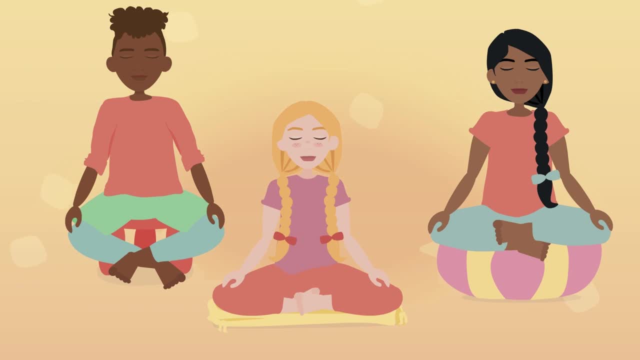 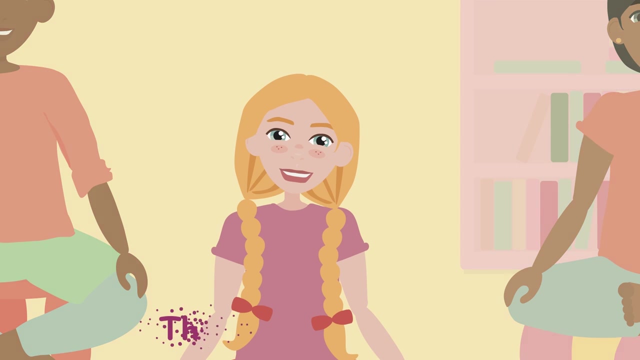 day. I am a hard worker, I can do hard things, decisions, things- and I am unique. I am a good person, I am loved. Take one last deep breath in and let it out Now, slowly open your eyes. Great job Now you're ready to have an amazing day. 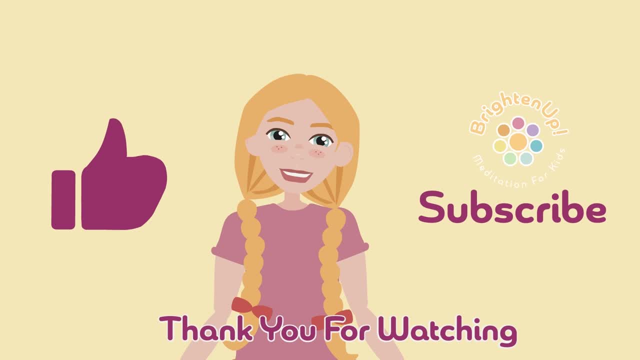 Thank you for starting your day with me today. If you like this video, please like and subscribe For more positive content.